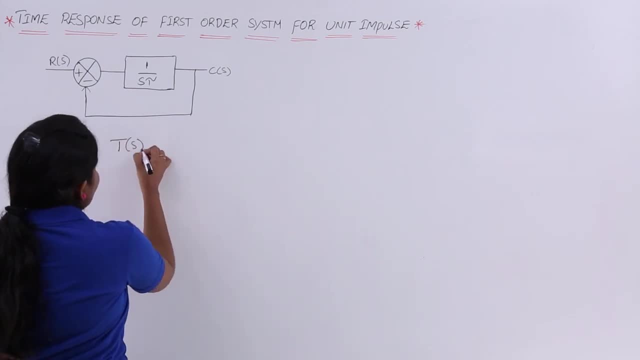 diagram. if you consider, the transfer function T of S is equivalent to C of S by R of S. So this is equivalent to: according to the negative feedback theory, we can write this: the transfer function of the system as g by 1 plus g h. 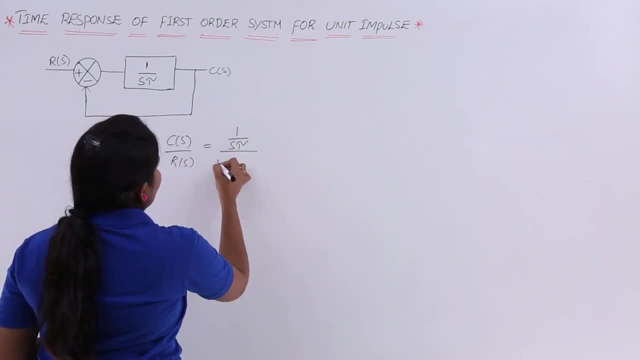 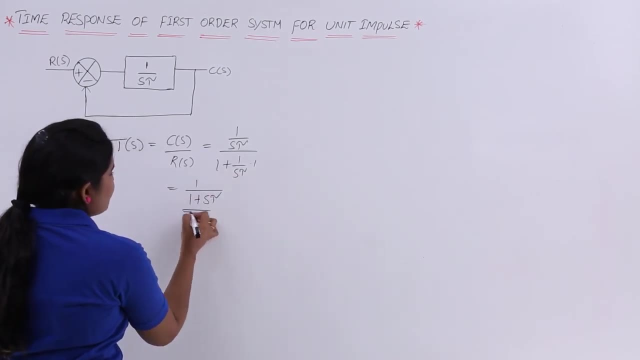 So that means 1 by S tau, divided by 1 plus 1 by S tau, into 1.. So this is equivalent to 1 by 1 plus S tau. you are going to get This is the transfer function of this first order system. 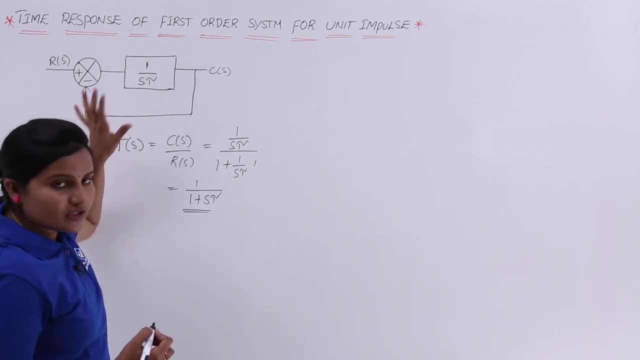 What we need to find out: time response of this first order system for the input as impulse. we need to find out. So here, time response is nothing but the response of the system in terms of time. So this is the time response of the system in terms of time. 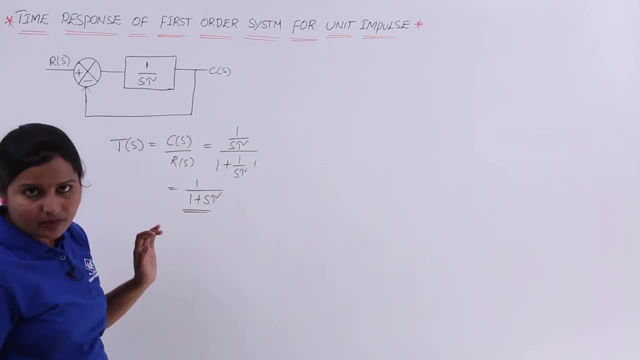 So this is the response of the system in terms of Laplace transform. So that means in terms of frequency or in terms of S domain. But we need to find out the response of the system, the output of the system, with respect to time. then we can say that response as time. 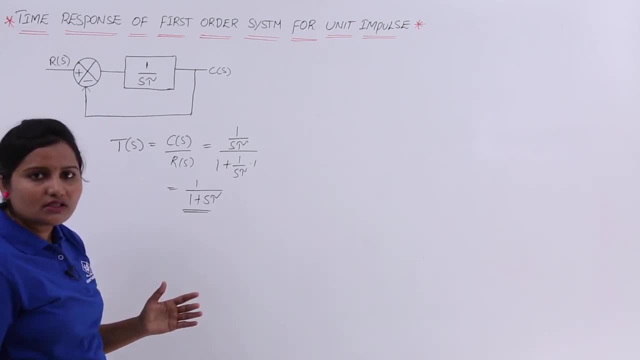 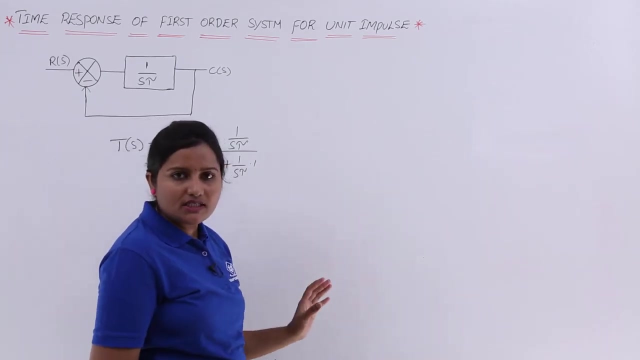 response. So to find time response of the system is nothing but finding the output of the system. Ultimately we need to find out the C of T. So here I am having my transfer function you just keep aside before getting into the procedure. I want 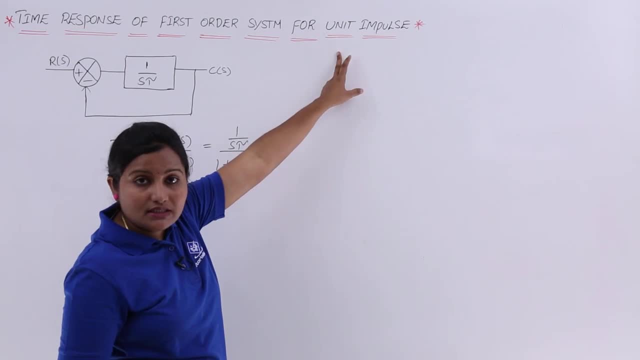 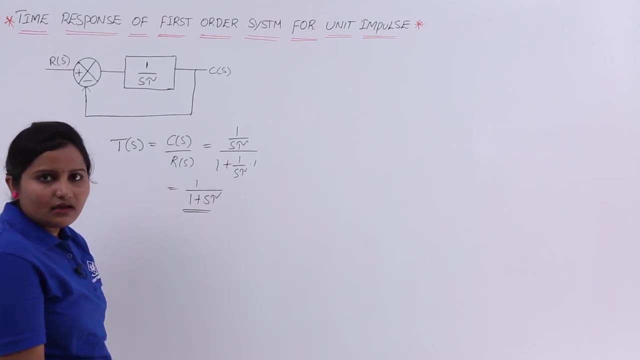 to discuss about my test signal. So here I want to consider unit impulse as my test signal, So that I need to apply as input to test the signal with that system. I need to apply that signal as input. So my R of T will be equivalent to impulse. So here R of T is equivalent to del of T. So 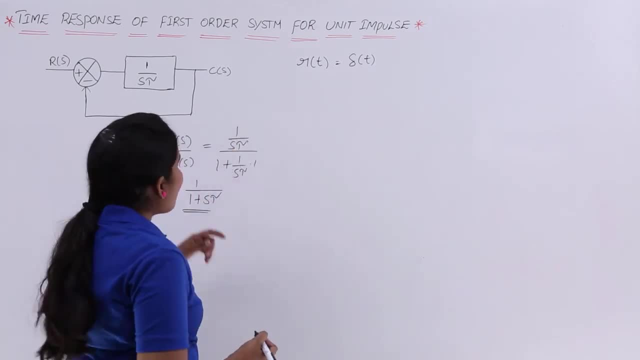 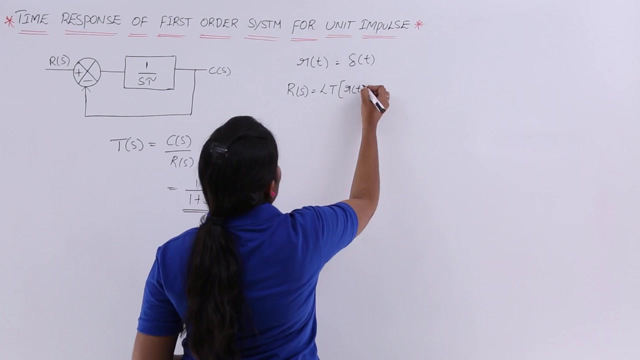 del of T I need to consider, but I want R of S. So our block diagram: if you observe our block diagram, that will be in S domain. So R of S is equivalent to: if you consider Laplace transform of R of T, then you are going to get R of S. That means Laplace transform of del of T. you 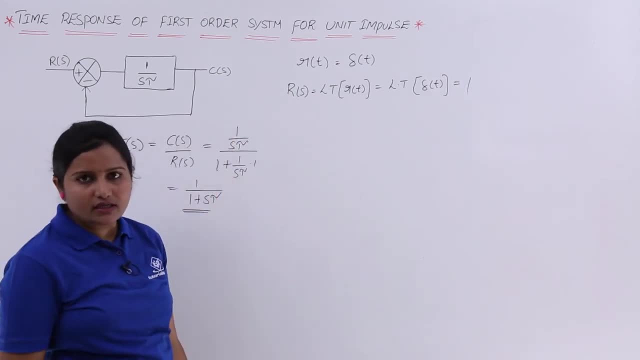 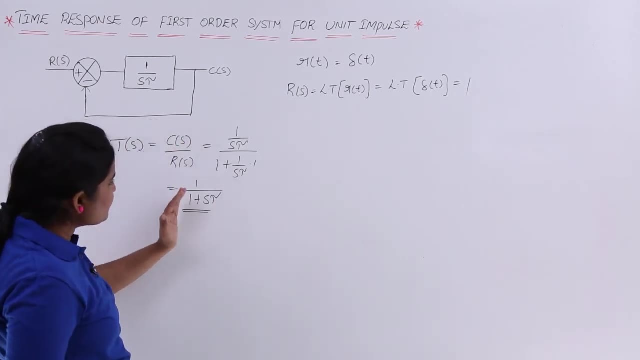 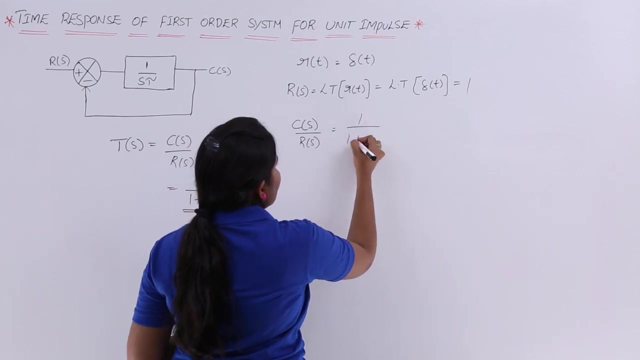 know that Laplace transform of impulse function is equivalent to 1.. Now I am considering this equation: T of S is equivalent to C of S by R of S. My transfer function, C of S by R of S, is equivalent to 1 by 1 plus S tau. This is my transfer function. I need to find out. 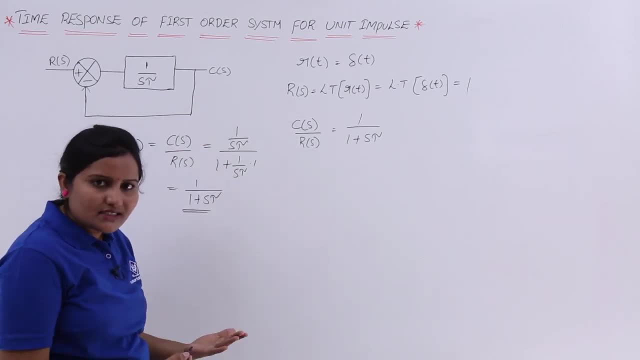 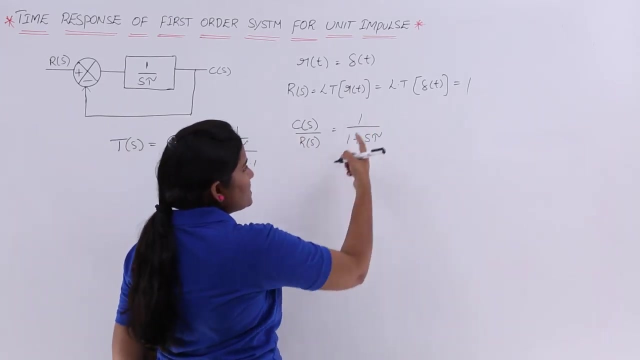 C of T. So what are? what is the way to find out that C of T means? first I want to find out C of S. after that I want to apply inverse Laplace transform. then I use it to get C of T here. So to get C of S. I am having this abstract. I am just sending this R of S to that side. 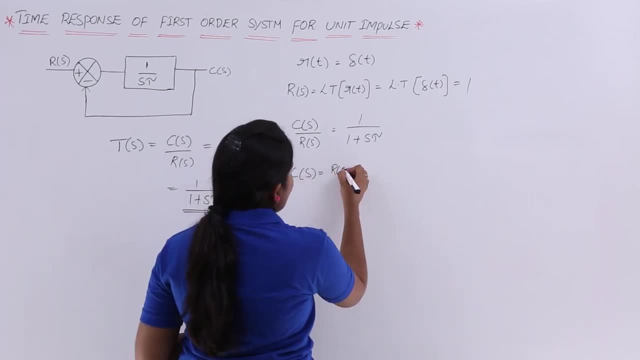 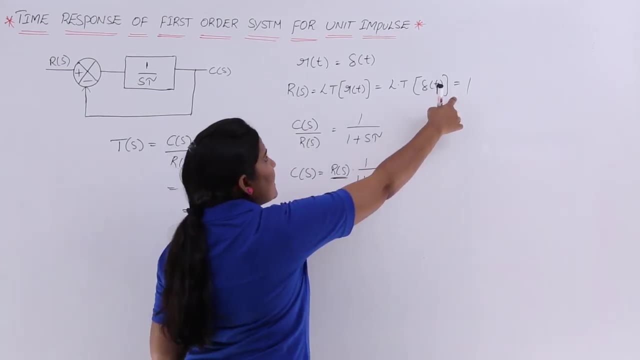 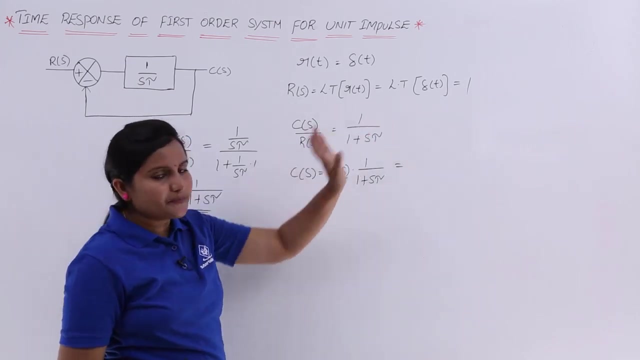 So then I will get C of S is equivalent to R of S into 1 by 1 plus S, tau, We know the value of R of S. So we are giving, as we are giving, unit impulse as our input. our transform of that input is equivalent to 1.. We already found that value. So here the resultant of: 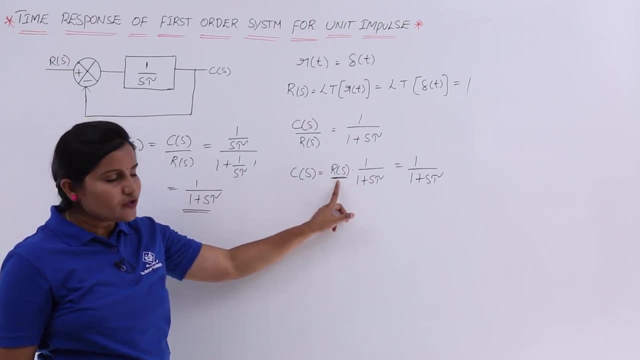 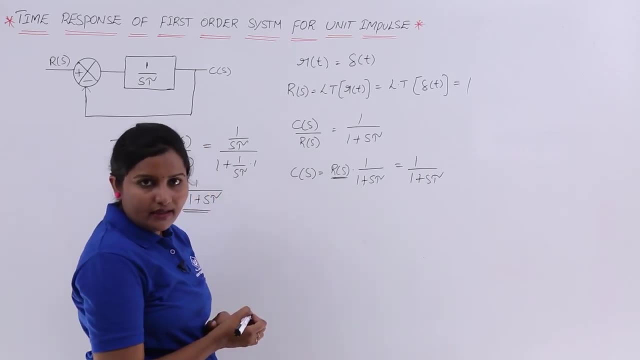 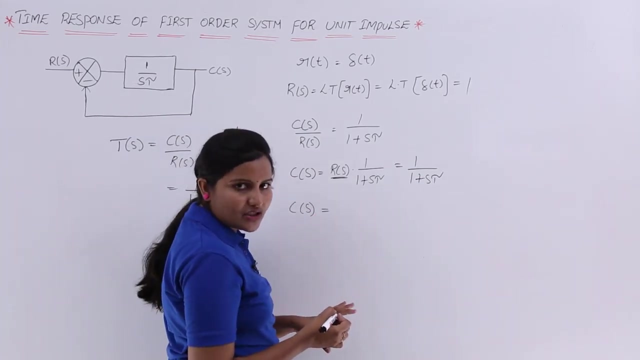 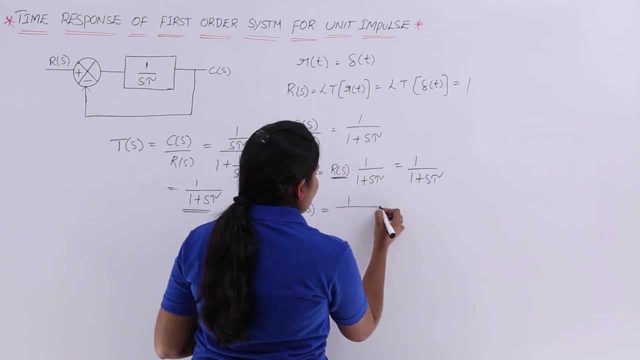 the C of S is approximately 1 by 1 plus S tau, So the divided by 1.. So that is 8.0 degrees, And C of S then is equal to 1 by 1 plus S tau. If you substitute R of S is equivalent to: 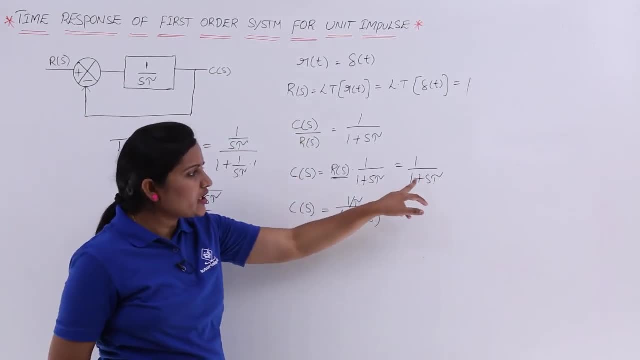 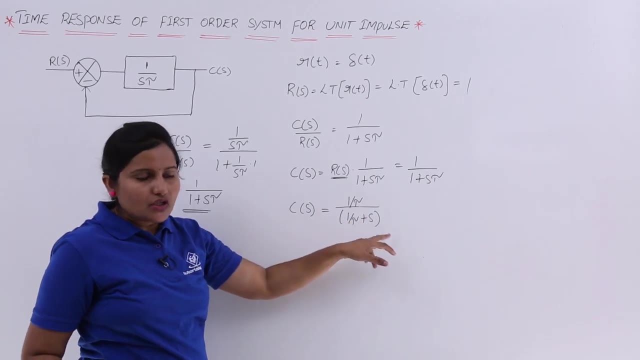 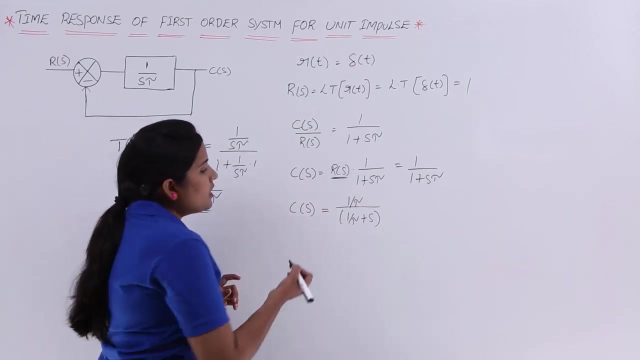 I am writing like this: You can see I am taking common of tau here, that tau I want to send to denominator. If I take in common of tau, you will get 1 by tau here. So I am writing this equation like this: If you modify you are going to get the same, And here, if you. 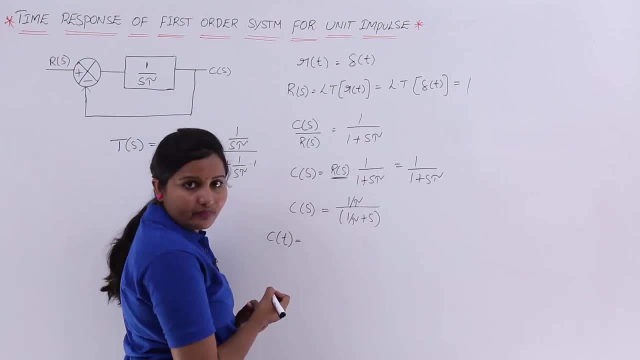 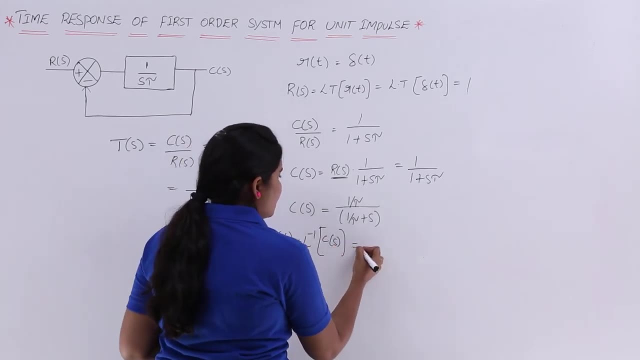 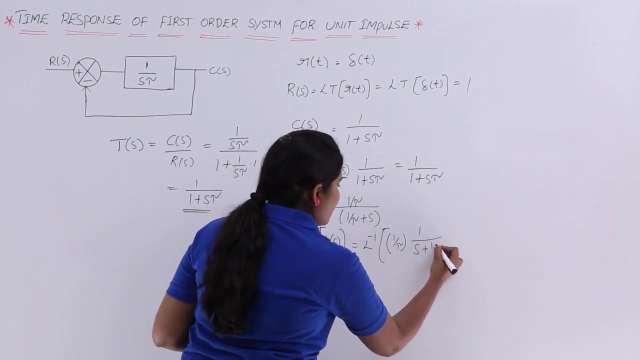 apply. if you want to find out c of t, then you need to consider the inverse Laplace transform of this c of s. That means inverse Laplace transform of 1 by tau is a constant and for remaining one s plus 1 by tau. So now this is, as this is a constant, the inverse Laplace. 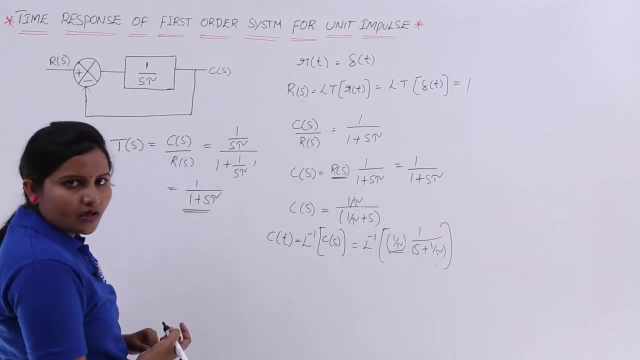 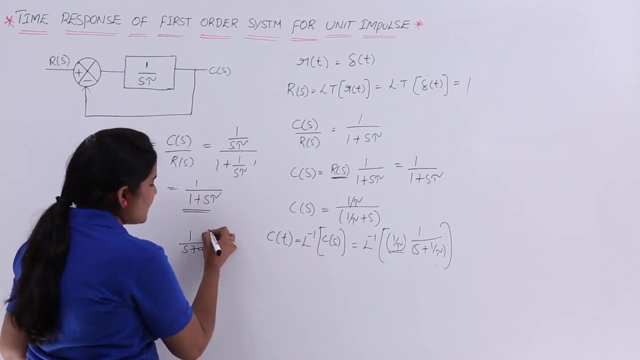